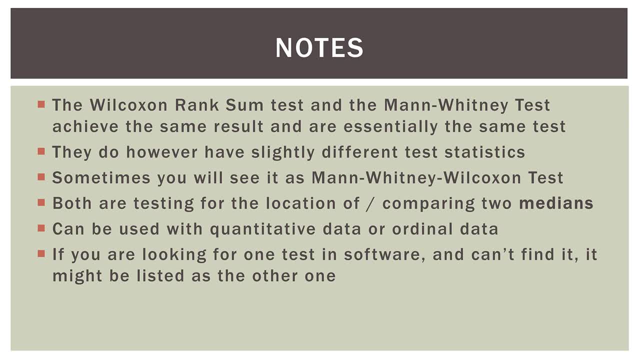 as the other test, so the Mann-Whitney test. It really depends on the software you're using. But just realize that the Wilcoxon Rank Sum test and the Mann-Whitney test are the same. they give the same result and sometimes 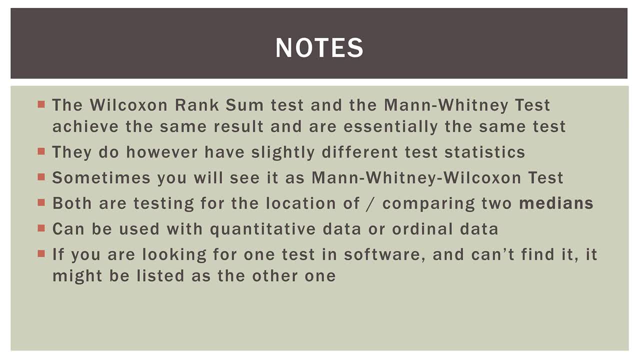 they're actually listed combined as the Mann-Whitney-Wilcoxon test Depends on the software and the book you're using. Now each test has its own set of subscripts and notation, so don't get confused. but in the end 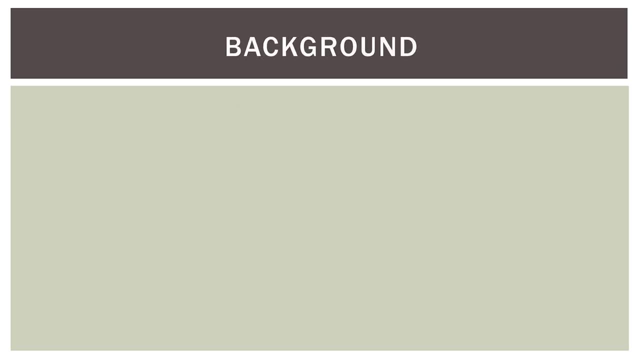 they're essentially the same test. So a little bit of background. So if we were doing a parametric version of this test for two samples, that will lead us to use the independent samples t-test. So the independent samples t-test is the first comparison test we learn about. 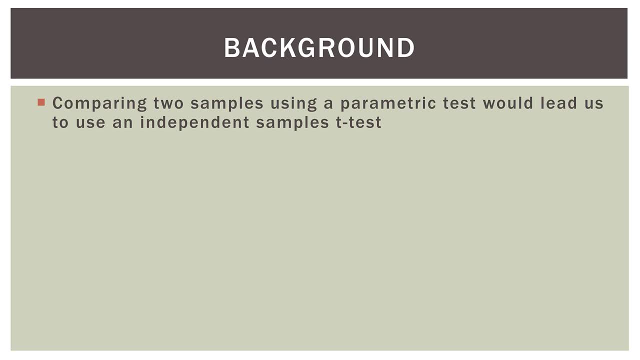 in basic statistics. In that test we are comparing the location of two means from two samples, and those samples are assumed to have normal distributions. So if you remember the independent samples t-test and the independent samples t-test, this is really the non-parametric version of that test. 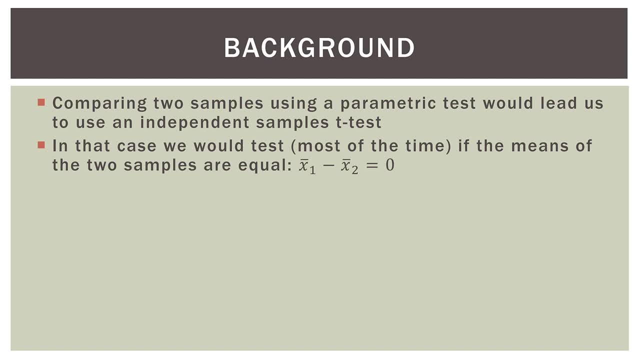 Now, in the case of that parametric test, the independent samples t-test, most of the time we will be comparing if the two samples are equal or the means of those two samples are equal. Now, another way of saying that is that the difference 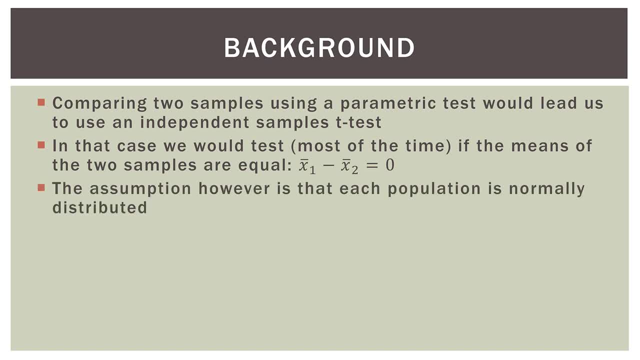 between those two means is zero. The assumption, however, is that each population is normally distributed. The Wilcoxon Rank Sum or the Mann-Whitney test allows us to compare two populations where the underlying distributions are not normal but do have similar shapes. 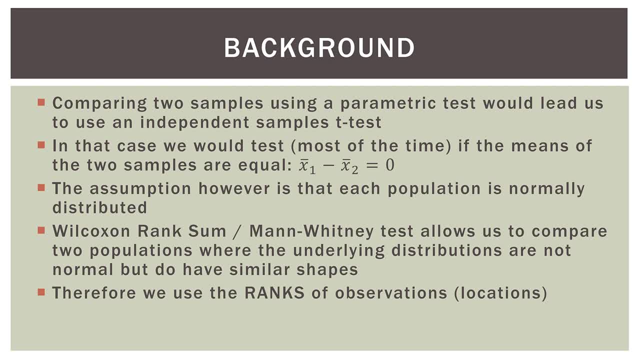 Now to do that, we use the ranks of our observations within the sample, not the actual underlying value. That's why it's called the Wilcoxon Rank Sum Test. We're gonna use the ranks, So we'll take our values, line them up. 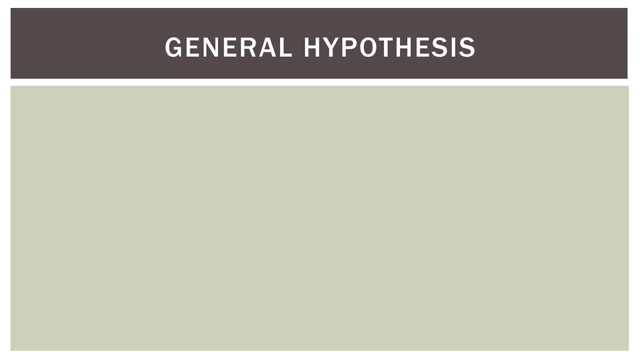 and turn them into ranks. So here is our general hypothesis. The null hypothesis states that the two populations are the same or the medians are in the same location. The alternative hypothesis states that the two populations are not the same or the locations of the medians. 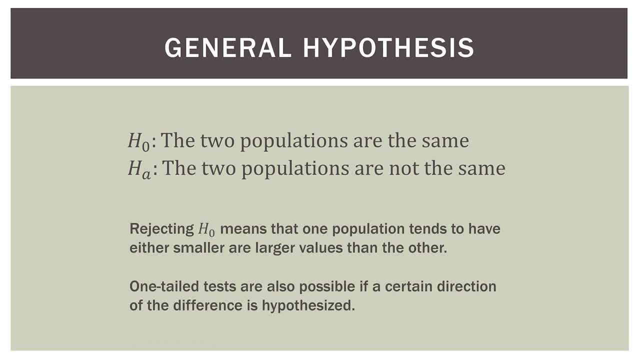 of the two populations are not the same, So rejecting our null hypothesis means that one population tends to have either smaller or larger values than the other. It really depends on what type of hypothesis we set up. Now. one-tailed tests are also possible. 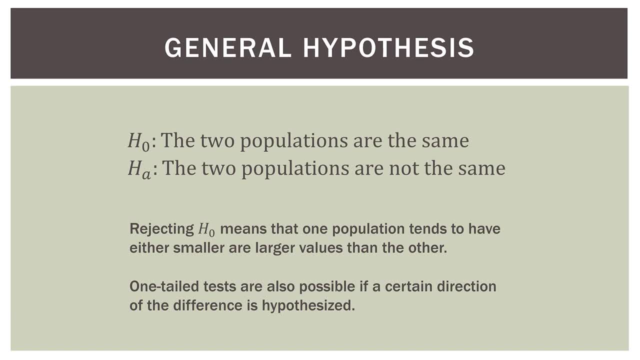 just like we have in the independent samples t-test we talked about before, If a certain direction of the difference is hypothesized. So we can say that the two medians are in the same location or are equal, or we can say that one median is above another. 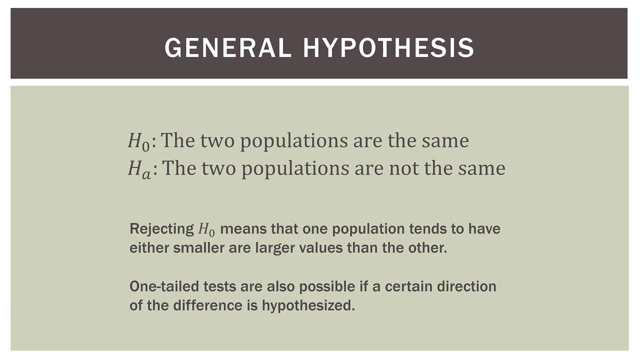 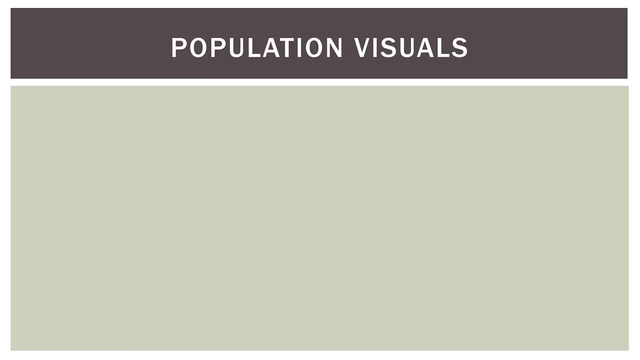 or we can say that one median is below another. All of those are possible in the Wilcoxon Rank Sum or Mann-Whitney Test. So let's go ahead and look at some visuals so you can envision this in your mind. So the first case, we have population one. 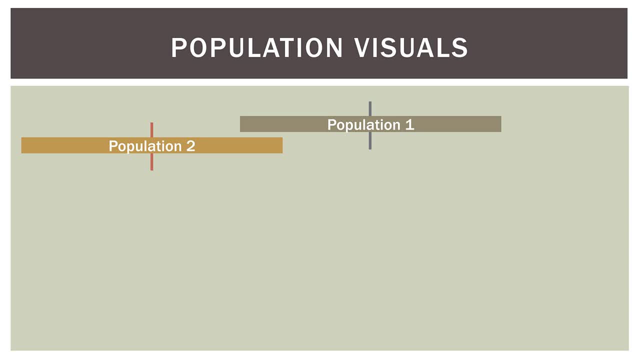 over here. on the right, it's median is denoted by the vertical line. On the left, we have population two and it's median is denoted by the vertical line. Now notice: there's not much overlap between these two populations. 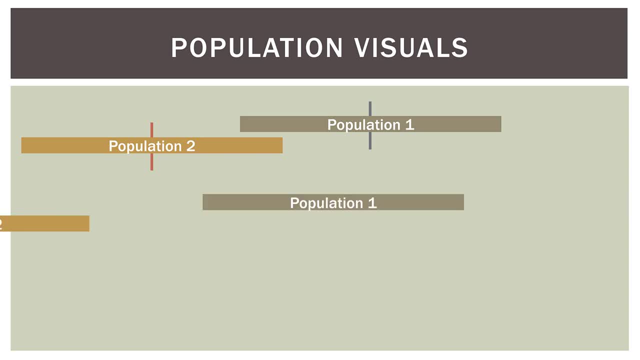 and the medians are pretty far apart. Now in this case the populations are a bit closer together, So there is a bit of overlap in the middle. The median for population one a bit closer in distance to the median of population two. 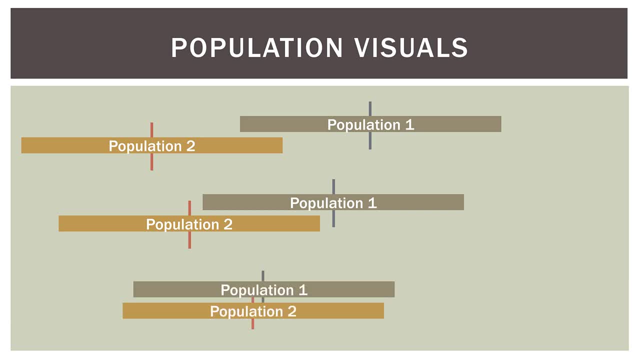 Now in this third example we can see that the populations are pretty much completely overlapping. The location of the median for population one and the location for the median of population two are very, very close. So here we can see three examples, starting with, the populations are very far apart. 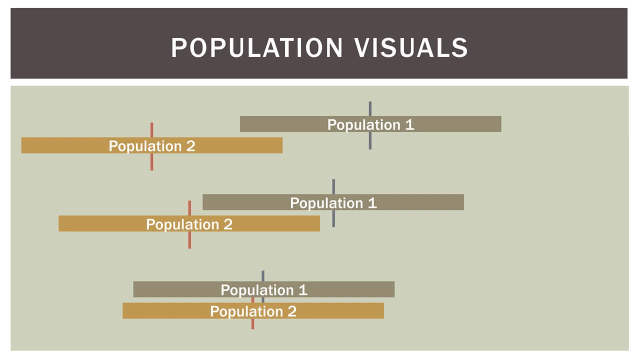 do not overlap and the medians have quite a bit of distance between them, all the way to the bottom, where the populations are overlapping and the medians are very close. Now, another way of thinking about this, in terms of our hypothesis, is this: 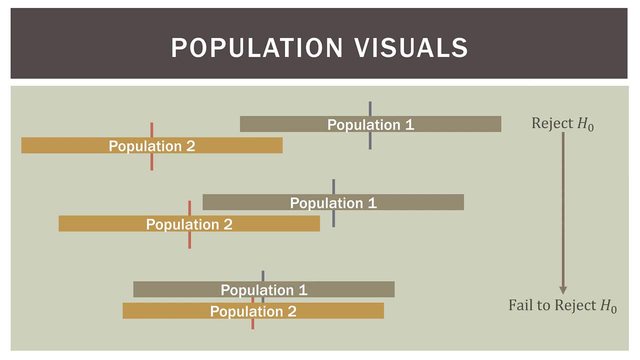 At the top, we would most likely reject our null hypothesis. Remember, the null hypothesis states that these two populations are the same, that the location of their medians are the same. Now, down below, we would probably fail to reject the null hypothesis. 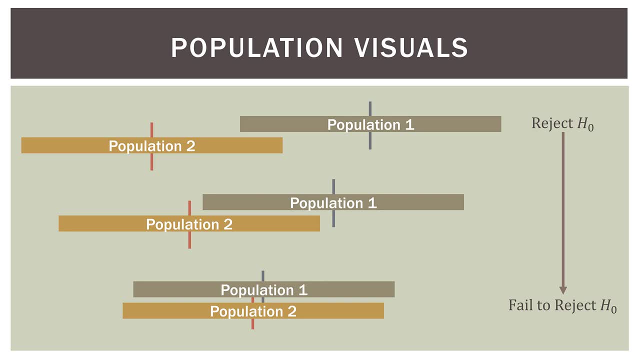 And that, of course, is because the populations basically overlap and the locations of the medians are very, very close to each other. So look at the visual over here in the left part of this slide and then match that to the hypothesis formulation. 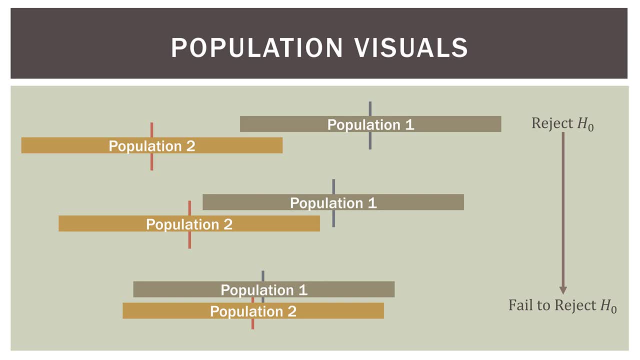 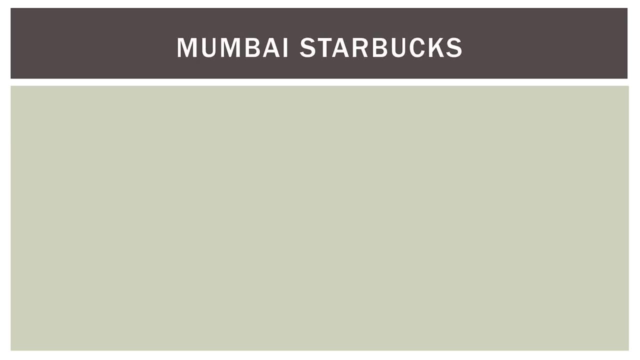 over here on the right So you can kind of see this in your mind how one relates to the other. Okay, so let's look at an example, without actually running the numbers. We'll do that in the next video, But here is sort of a problem. example of how this works. 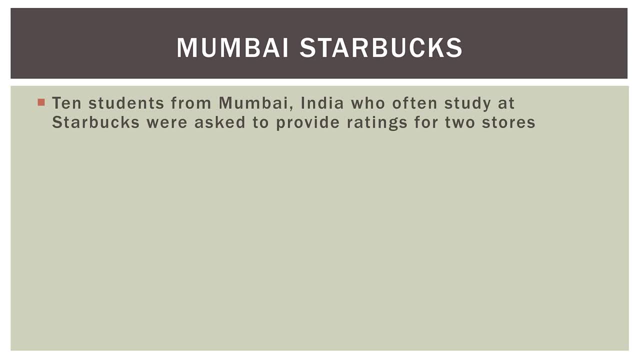 We'll call it the Mumbai Starbucks. So 10 students from Mumbai, India, who often study at Starbucks, were asked to provide ratings for two stores. Five students were asked to review the Churchgate store, which we'll denote with the letter C. 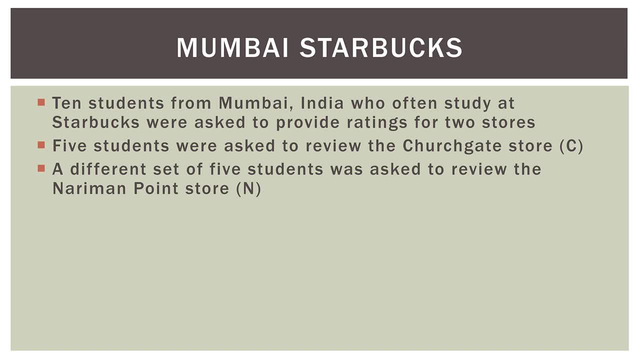 A different set of five students was asked to review the Netterman Point store, which we'll use the letter N to denote, And the survey covered five criteria: cleanliness, service facilities, drink quality and food quality, each on a scale of one to five. 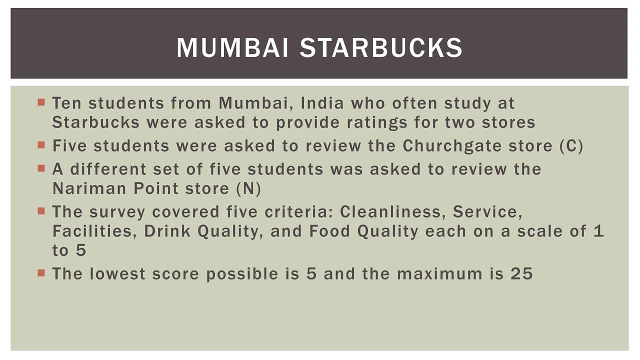 So, therefore, the lowest possible score is five. So if one of the stores got a one on all of these criteria, that would sum up to five, And the maximum is 25.. So if another store got a five on each of the five, 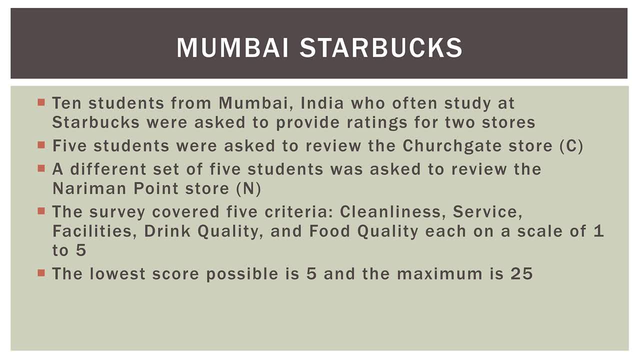 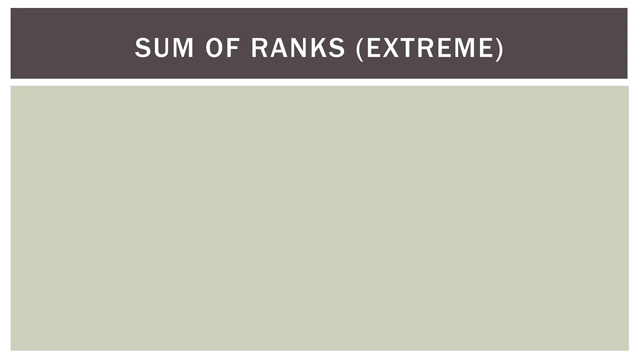 categories, those would sum to 25.. However, the score itself is not really important. What we're looking for is the rank. We're gonna compare the ranks of the scores, So let's take an extreme example, just for the sake of it. 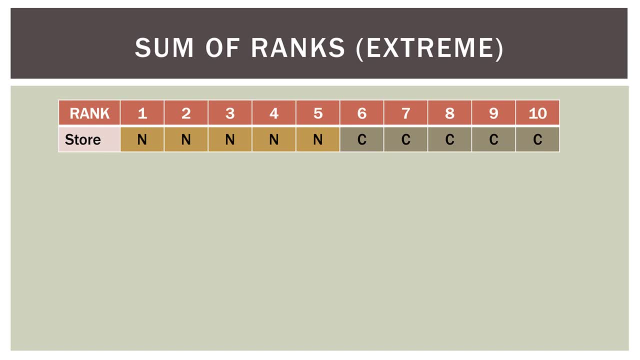 just for the sake of learning, Let's say it turns out like this. So for the first five ranks, if we put all the scores in order, the first five ranks are occupied by the Netterman Point store. So rank one, two, three, four and five. 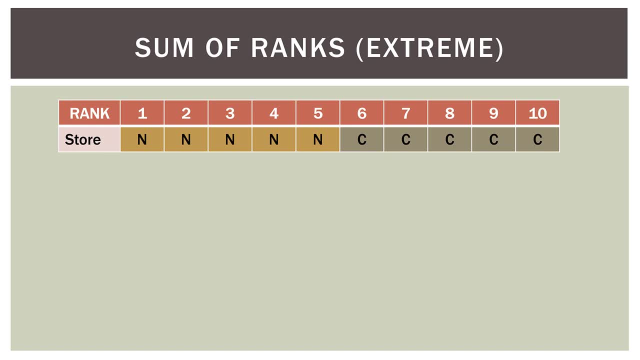 And then the final five ranks are occupied by the Churchgate store. So six, seven, eight, nine and 10.. Now what we do is we sum the ranks, Hence the Wilcoxon rank sum test. That's in the name. 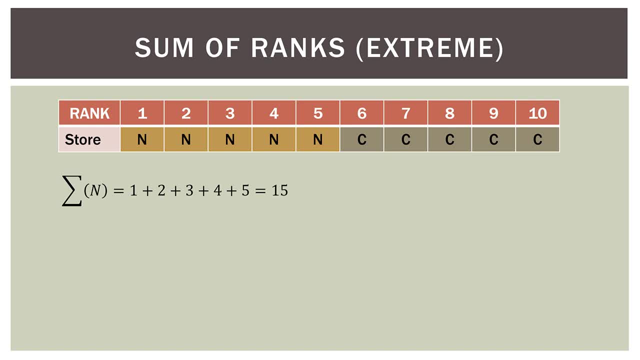 So for Netterman Point, we sum one, two, three, four and five. We have a total sum of our ranks which is 15.. For the Churchgate store we do the same thing, So six, seven, eight, nine and 10.. 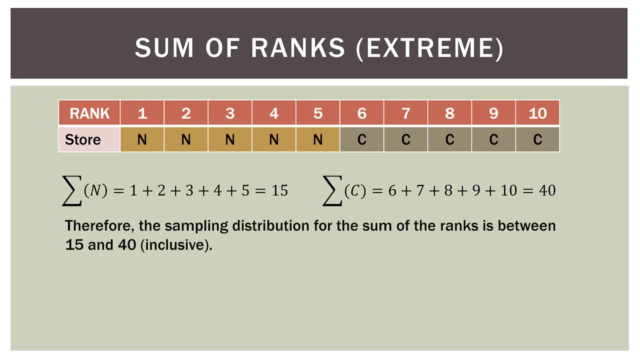 So the sum of those ranks is 40. Therefore the sampling distribution for the sum of the ranks is between 15 and 40. So the lowest possible sum of ranks we can have here is this case: one, two, three, four, five or 15.. 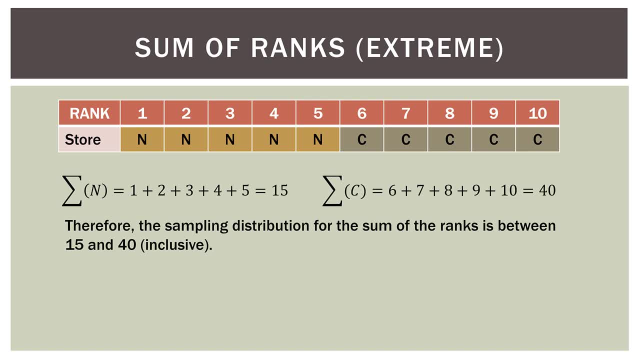 The maximum sum of ranks we could have in this situation is six, seven, eight, nine and 10,, which is 40. And that is the range of our sampling distribution. Now, this is important If the populations for each one of these stores is the same. 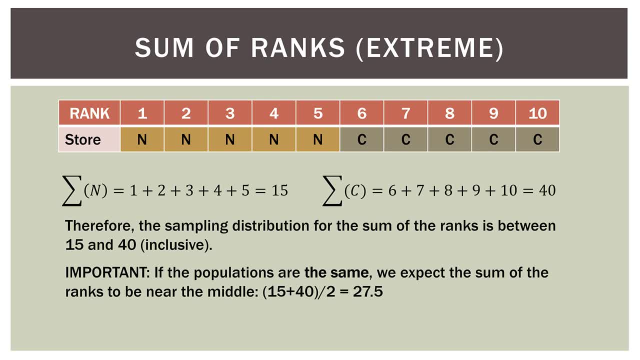 in terms of their scores and their ranks. we would expect the sum of the ranks to be near the middle. So in the low end we have 15.. On the high end we have 40. The middle of those two numbers is 27.5.. 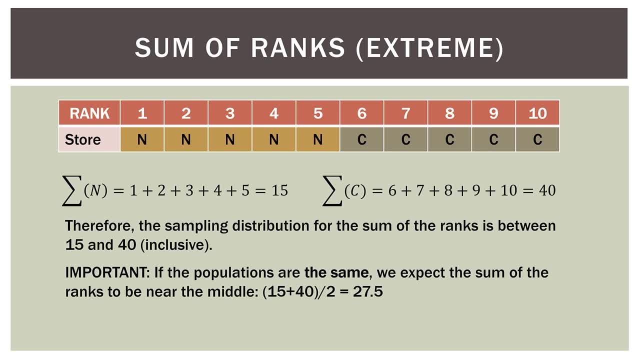 So if the stores overlap in their ranks, or if they overlap in their visual distribution, we would expect the sum of the ranks to be near 27.5.. But in this case we have one extreme of 15, the other extreme of 40.. 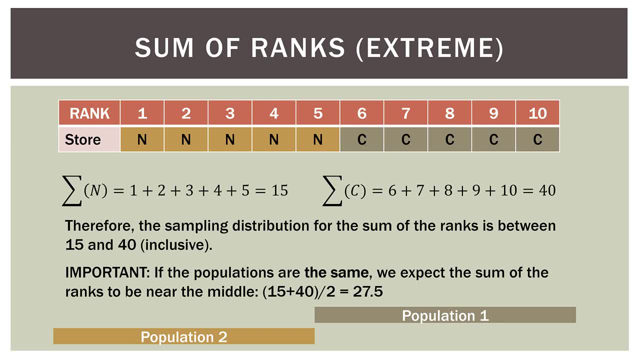 So therefore it would look something like this visually: So all of Churchgate's ranks are on one side, All of Ninnerman Point's ranks are on the other side. There is no overlap at all and therefore we would reject the null hypothesis. 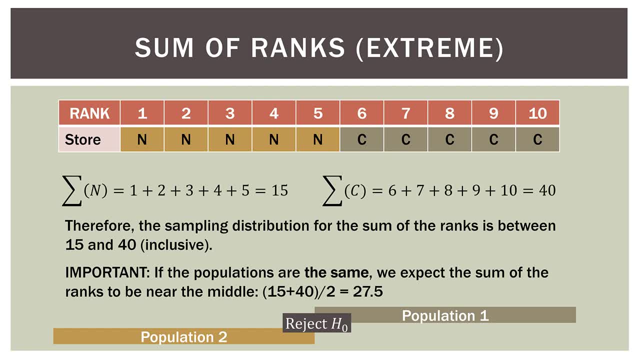 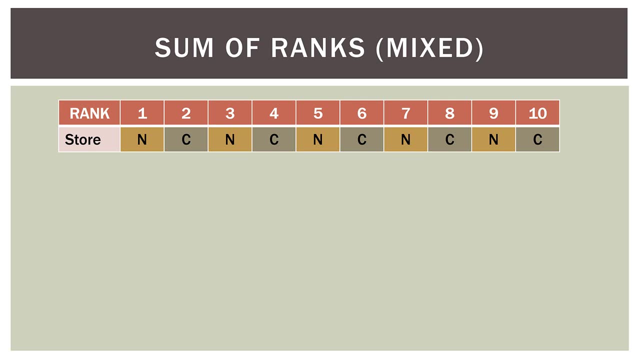 Remember, the null hypothesis states that these two populations are equal. Well, in this case, they are obviously not equal. They don't even overlap at all in this case. So now let's examine the other extreme, where the ranks are mixed. So in this case, we can see that each store alternates. 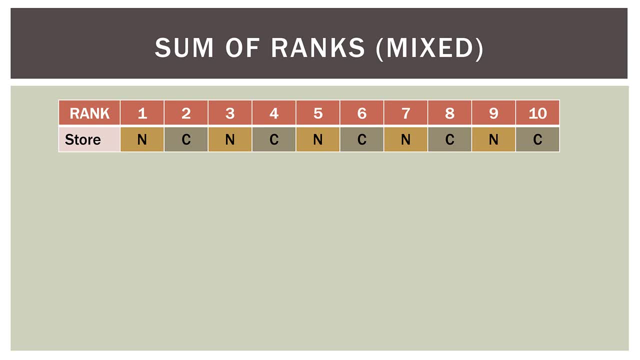 in terms of the rank. So we have Ninnerman Point in rank one, Churchgate 2, and then Nederman Point, Churchgate, so on and so forth. all the way down are 10 observations. So in this case for Nederman Point it's 1,, 3,, 5,, 7, and 9.. 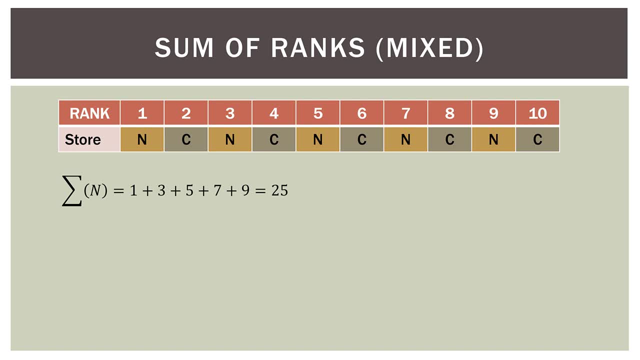 The sum is 25,. the sum of the ranks is 25.. For Churchgate, it's 2,, 4,, 6,, 8, and 10.. The sum of the ranks is 30. Now remember if the populations are the same. 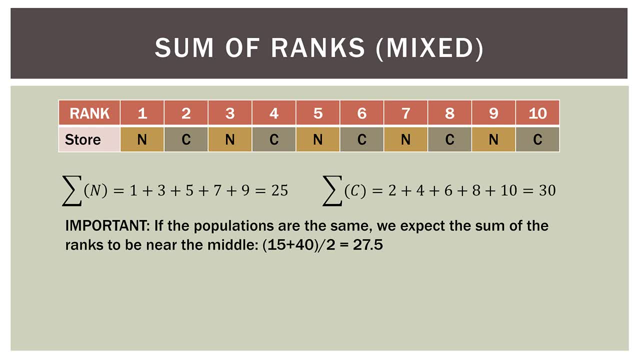 we would expect the sum of the ranks to be near the middle, which in this case is 27.5.. Well, in this case, this is as close as we can get, So alternating 1,, 3,, 5,, 7, and 9. 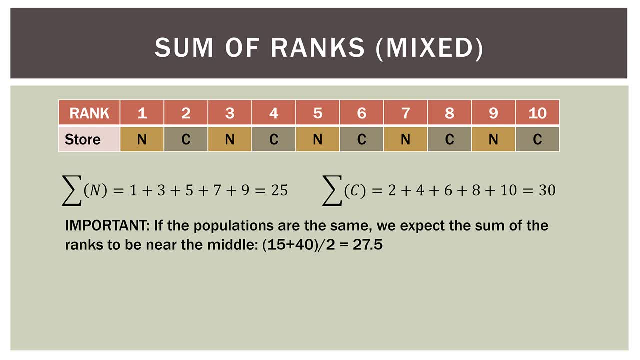 gives us a sum of rank of 25.. The other side 2,, 4,, 6,, 8,, 10, a sum of rank of 30. That's the closest we're gonna be able to get in this situation to 27.5, which is actually the middle. 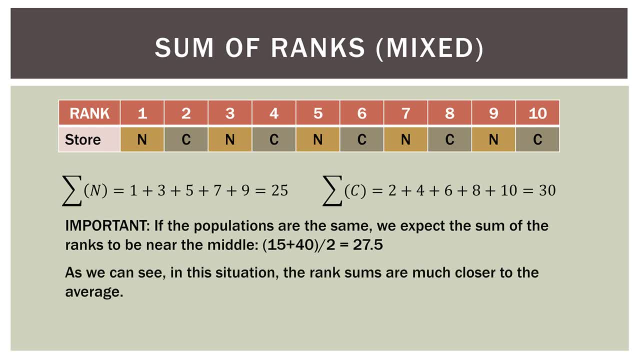 So, as we can see, in this situation the rank sums are much closer to the average if we average the rank. So let's look at the rankings together. So the populations look like this: We have Nenerman, Point slightly to the left. 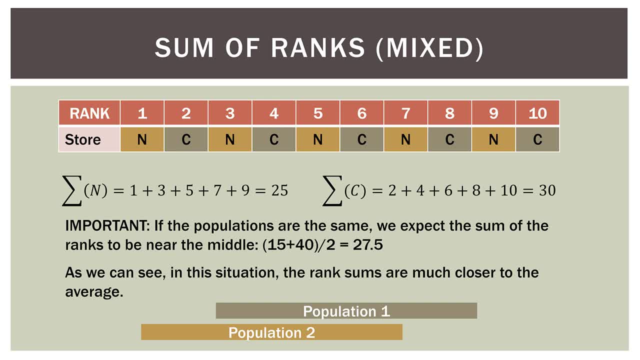 because it begins with rank one. Then we have Churchgate, slightly offset to that because it begins on rank two and therefore they overlap quite a bit. So in this case we would probably fail to reject the null hypothesis. So our null hypothesis states that these two populations 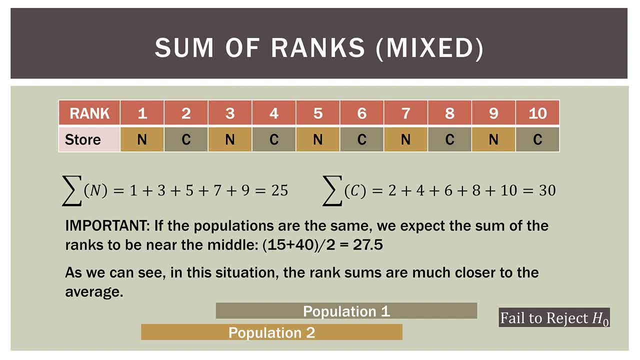 or these two stores are the same, The median location is the same And we can see here, at least visually and mathematically, that because they overlap so much that these probably come from the same population and there is no difference between the rank sums. 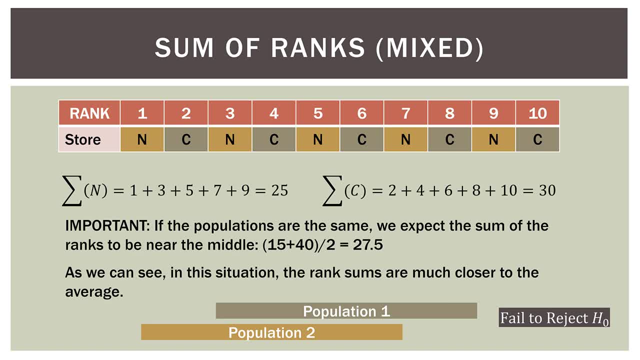 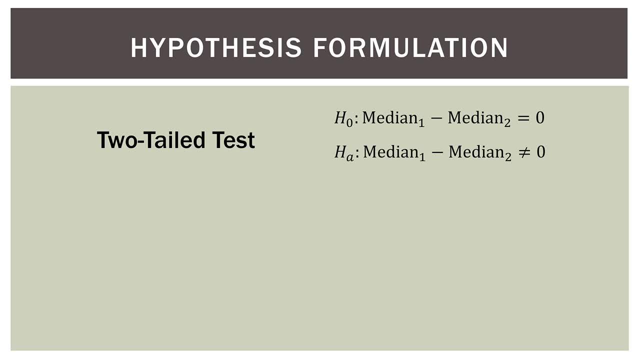 of Nenerman Point and the rank sums of Churchgate. So again we can have different hypotheses in the situation. So we can have a two-tailed test where we think the difference between the medians is zero. We can have a lower-tailed test. 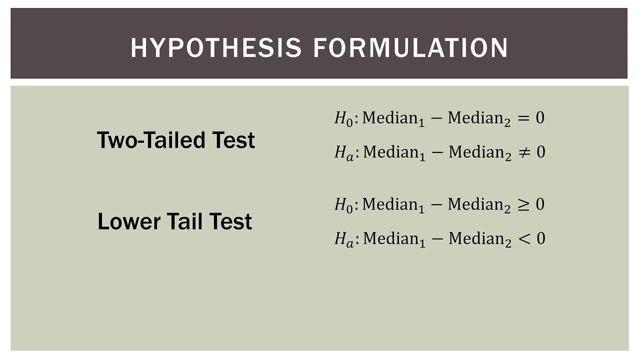 where the difference between the medians is greater than or equal to zero. The alternative would be the opposite. so less than zero And remember from way back when. the little trick to remember is that the alternative hypothesis points in the direction of your test. 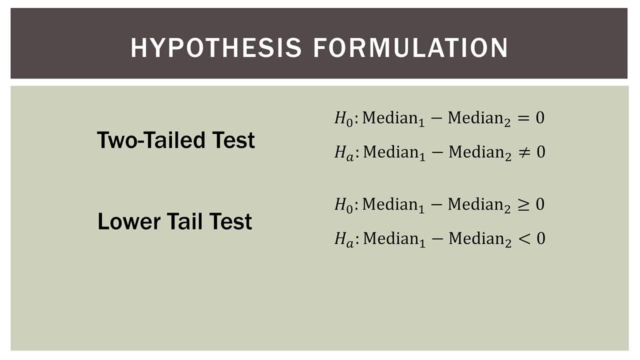 So this is a lower-tailed test. Therefore, we have the less than sign that's pointing to the left and that's how we can remember it's a lower-tailed test. Upper-tailed test is the exact opposite, So we can have the null hypothesis. 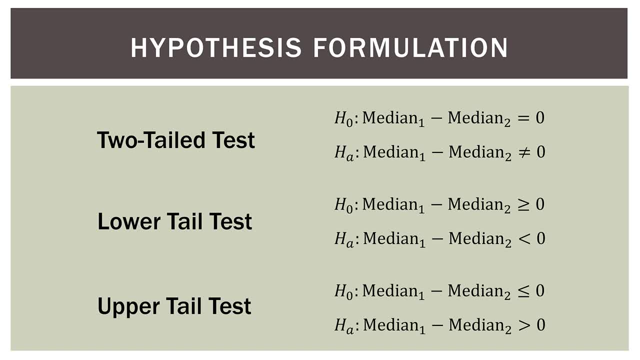 is that it's less than or equal to zero, and the alternative hypothesis is that it's greater than zero. So the sign is pointing to the right, the greater than sign. Therefore we know it's an upper-tailed test In the Wilcoxon rank sum and the Mann-Whitney test. 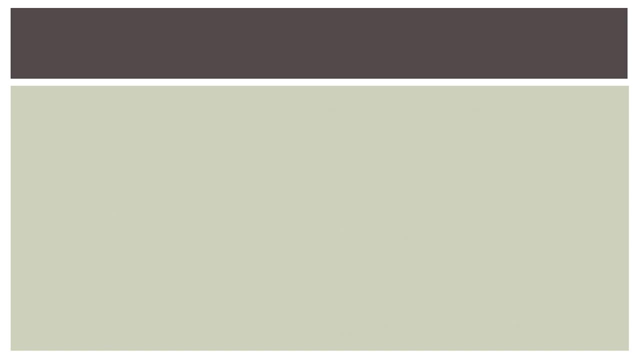 we can do any of these situations. Okay, so last slide of this presentation: How do we do this step-by-step Now? to keep this video reasonable in length, I went ahead and split it up into two parts, So this was the conceptual background. 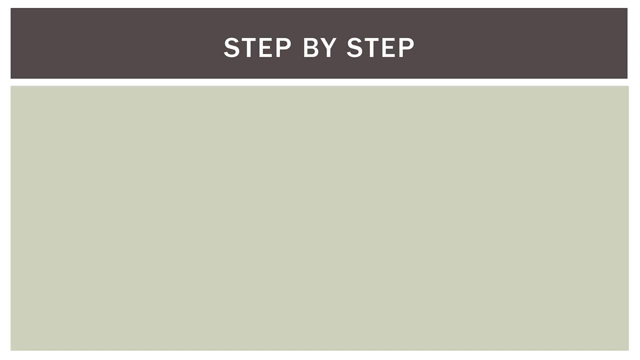 and the next video will actually go into Excel and I'll show you manually how to do this step-by-step. So how does it work? First, we place our samples into two columns, So in this case it would have been Nenerman Point and Churchgate. 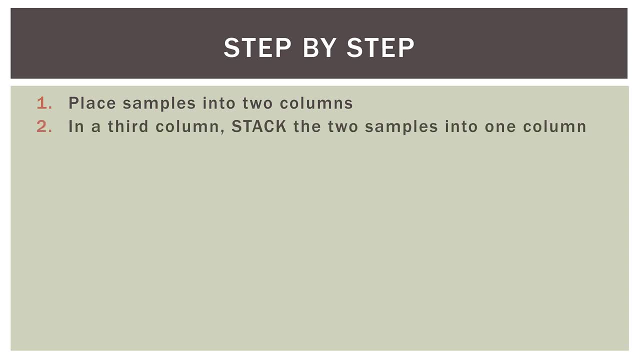 We put those in two separate columns. In the third column we then take those two samples and we stack them on top of each other into one longer combined sample, so into one column. In the fourth column we then rank each value in the stacked column. 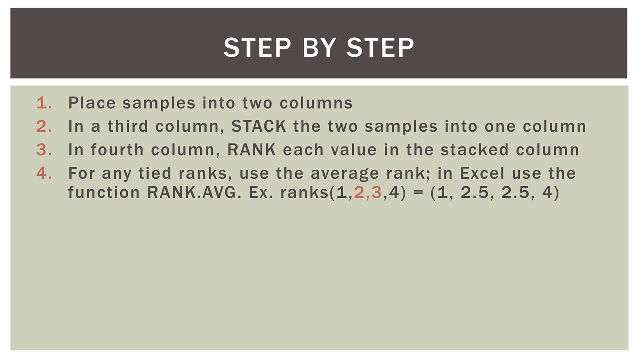 Now, for any tied ranks, we use the average rank, And luckily Excel has an actual function for this. it's called rankavg, or rank average, And here's how it works. Let's say we have four numbers, So the first rank and then the second. 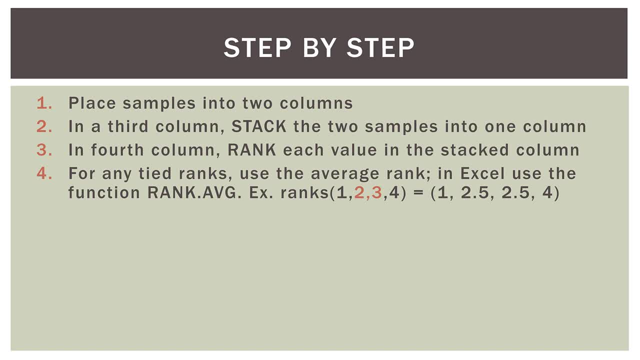 third and fourth numbers. Let's say, however, that the second and third numbers are the same. they tie. So one is not the second rank and one is not the third rank because they're the same number. In that case, we take the average of those two numbers. 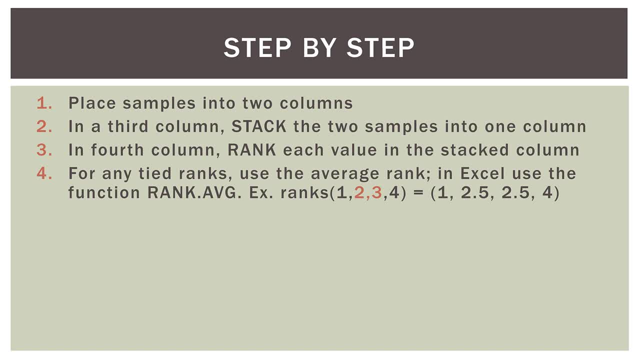 So for those four numbers the ranks would be actually one, 2.5,, 2.5, and four, And that's what the average rank means and that's what the rankavg function does in Excel, And again we'll see this in practice in the next video. 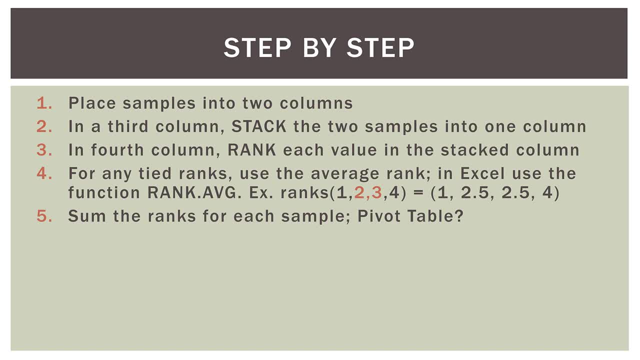 Then we sum the ranks for each sample. You could do that manually, you could do that using an if function in Excel, you could do that using a pivot table- whatever suits you. But we sum the ranks that belong to each sample individually and separately. 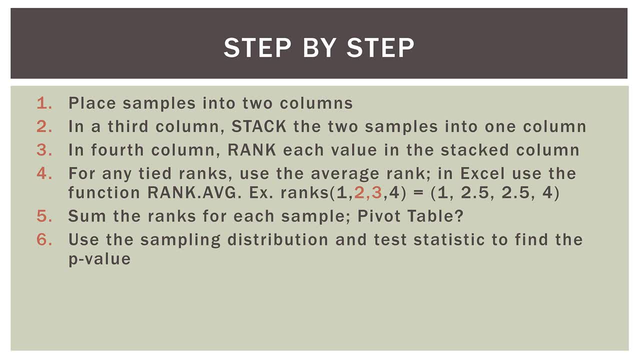 Then we use the sampling, distribution and test statistic, which we'll learn about in the next video, to find the p-value, Again very similar to how we do it in parametric statistics. Then we compare that p-value to our chosen alpha level.